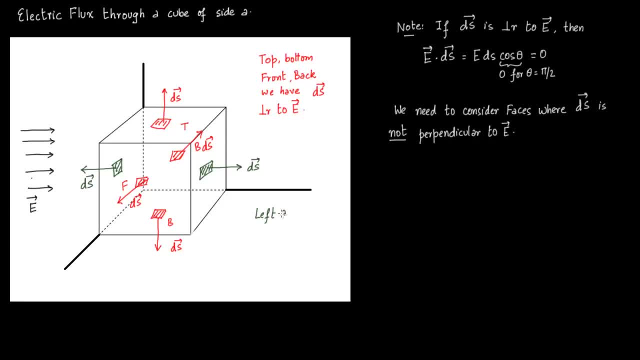 So here the ds vector is not perpendicular to the electric field. So left and right face will have non-zero flux because they are not perpendicular to the electric field. So let us start with the left face. So the flux is given as the surface integral of E vector. dot product with ds vector. 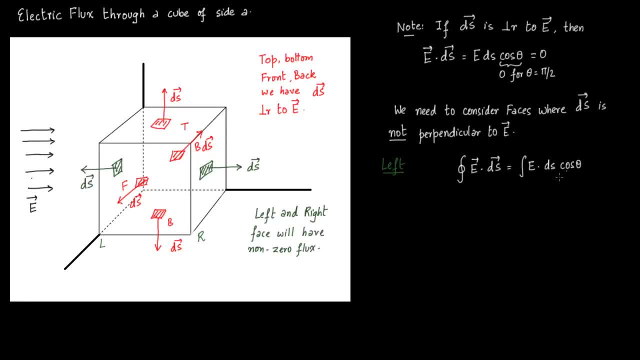 So this is E ds cos theta Notice that we are talking about the left face. So ds vector and E vector are pointing in opposite directions, So the angle between them is 180 degrees. So again, we are talking about the left face. 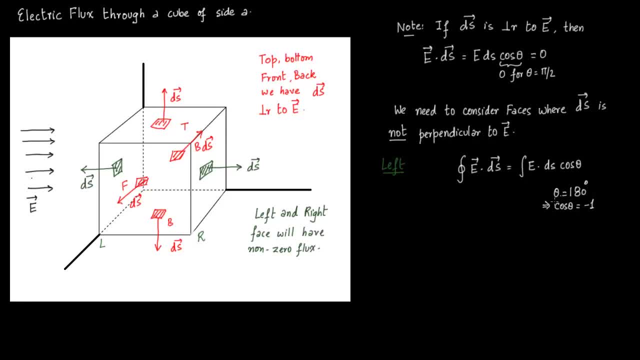 ds vector and E vector are pointing in opposite directions, So angle between them is 180 degrees. That means theta is minus 1.. So the integral now becomes minus E- ds. Since E is independent of the surface area, you take minus E outside and then you integrate. 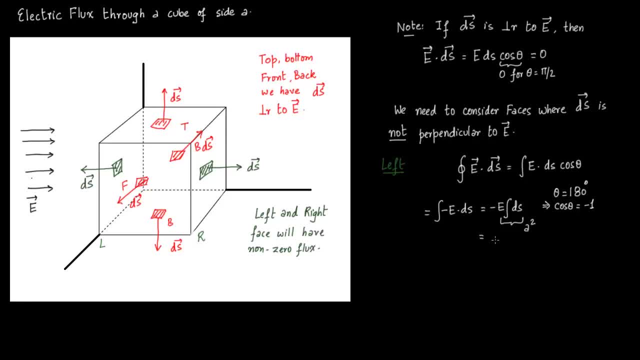 over the surface area. So since this is a cube of side A, the left face has area A square. So we have computed the flux through the left side. It is minus E A square, where A square is the area of the left face. 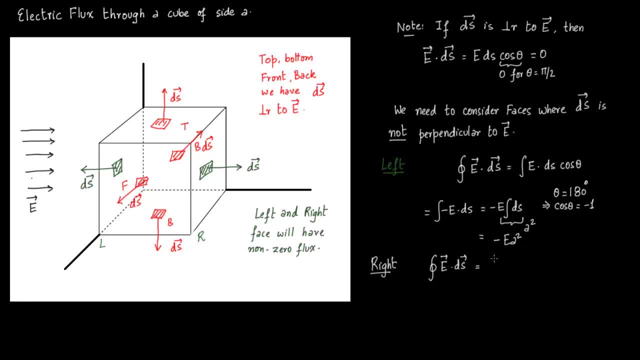 Now we talk about the right face Again. we copy down the formula of flux, which is surface integral of E vector, dot product with ds vector. This is equal to E, ds cos theta. Now ds vector and E vector are pointing in the same direction. 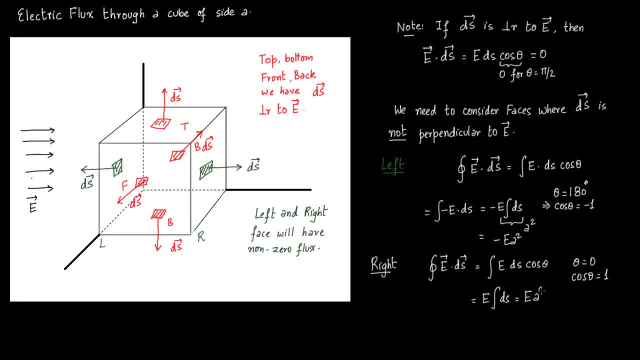 So, since they are pointing in the same direction, theta is 0.. So therefore, cos, theta is 1.. So you get E integral of ds, which is equal to E A square. So what is the net flux? So now, net flux is sum of all four faces. 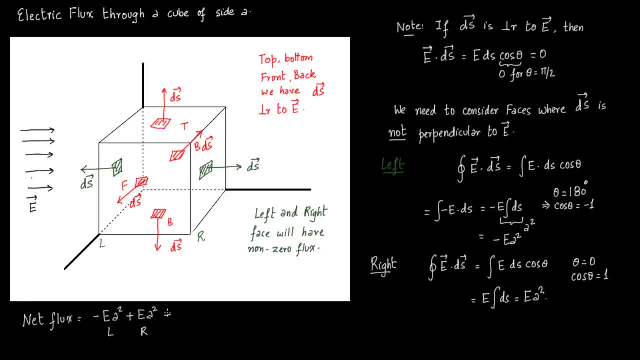 So you take left face plus right face, minus E A square plus E A square. Then you take top face, bottom face, front and back. All of those have 0 flux because their surface area is perpendicular to the flux. So even if you calculate the integral, you will take theta as pi by 2..